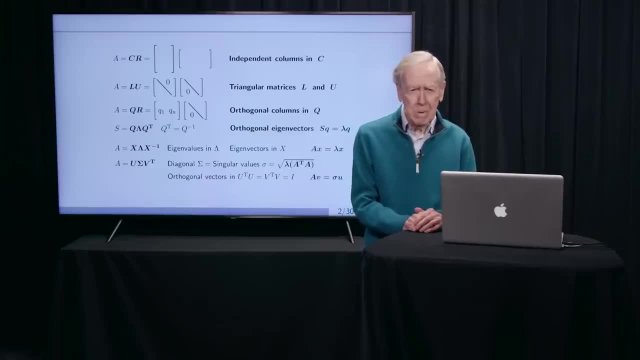 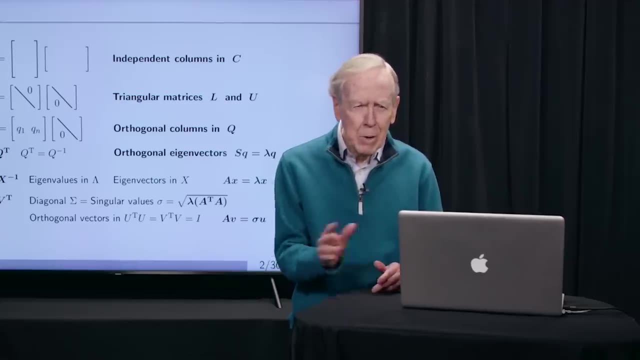 And so I wanted to say something about those later steps. And also, when I teach it now, I have a new starting point. 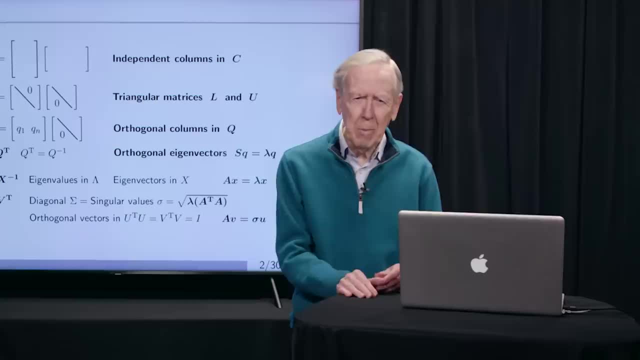 And I'll show you that. So I'll go a little slowly on that starting point. The slides tell you the whole course. And that's like crazy to have a full course within a short video, but especially 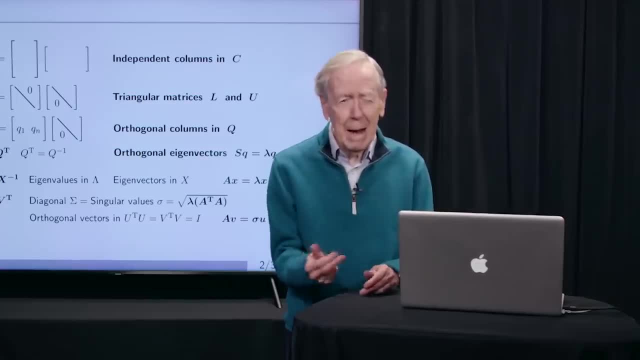 the first part is new. And I'm even writing a textbook called Linear Algebra for Everyone that will start this way. 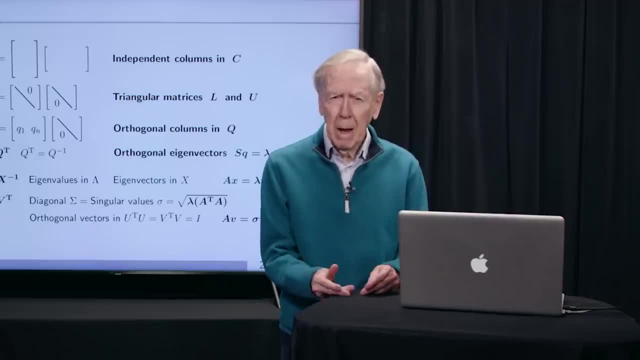 I hope that the new start brings in sort of real linear algebra ideas right away. 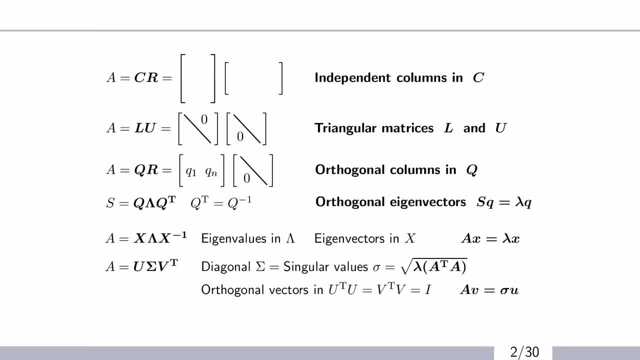 And let me show you where those are. So this is an outline of the whole video. And the first line. Which I think about in my mind as a matrix A is a product of a C matrix, a column matrix, and a row matrix R. And you'll see what those are. 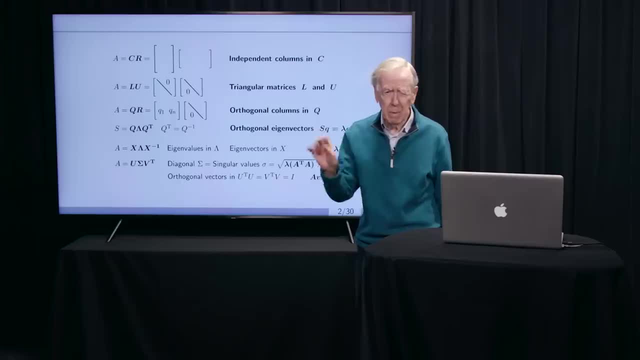 So that's the new idea. 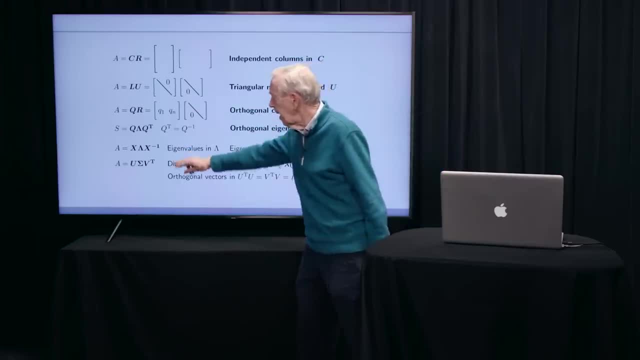 That will come first. Then these are five famous essential shorthand descriptions 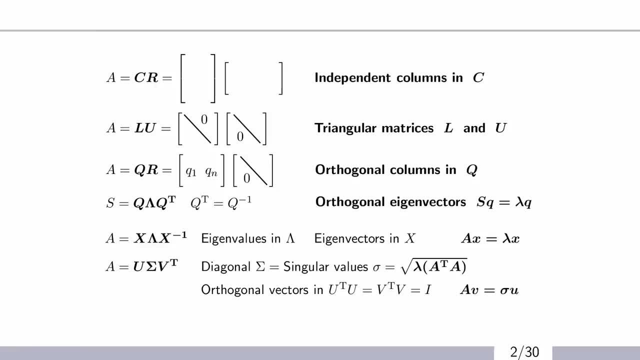 of the key chapters of linear algebra. The key chapters. 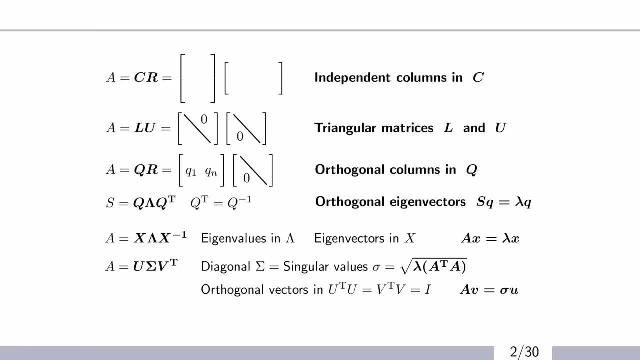 So they represent, for example, LU, as those letters are famous. And computer commands would be exactly those letters, LU, for elimination, for solving equations. The first job of linear algebra. And then QR. 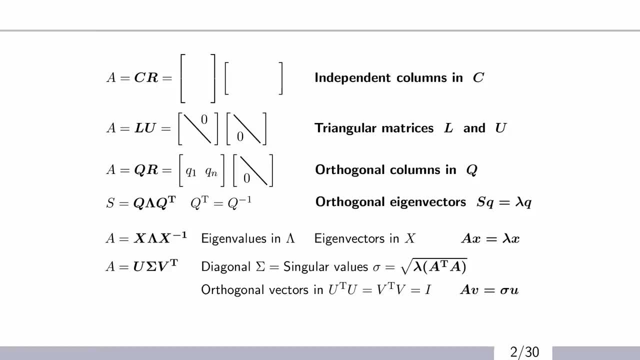 So Q is a very interesting, important type of matrix. That's standing for an orthogonal matrix. There's the word orthogonal or perpendicular. 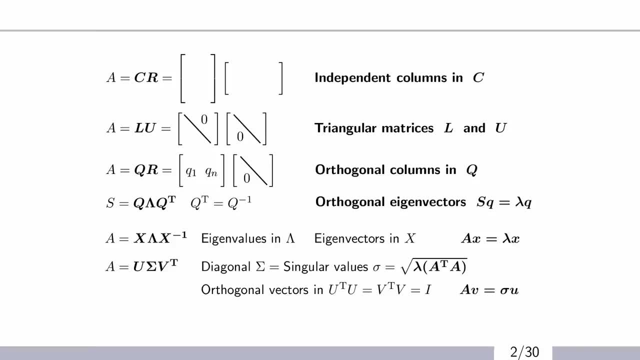 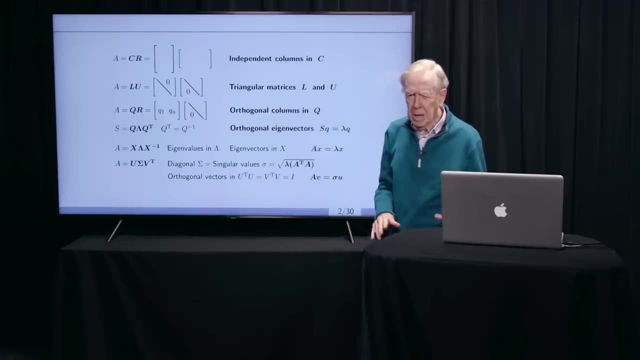 So those are the best matrices to compute with. And that QR gets us there. And S is for a symmetric matrix. And it will involve, oh, well, I should say the first half ending with there, with QR, is about solving equations.